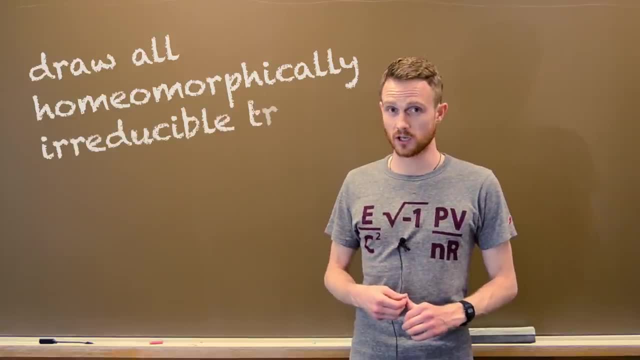 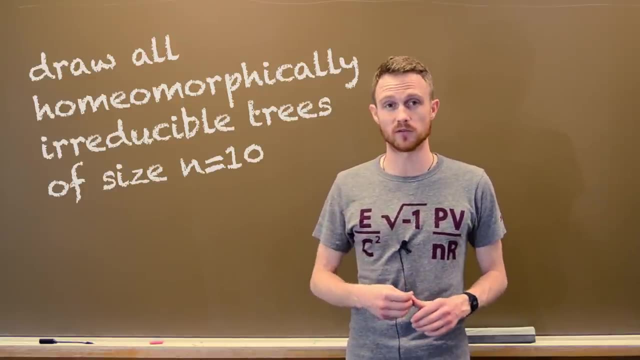 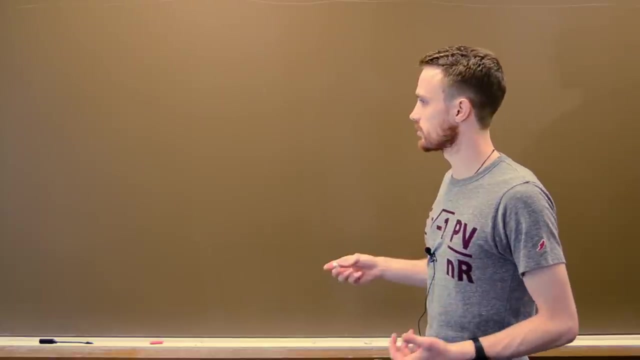 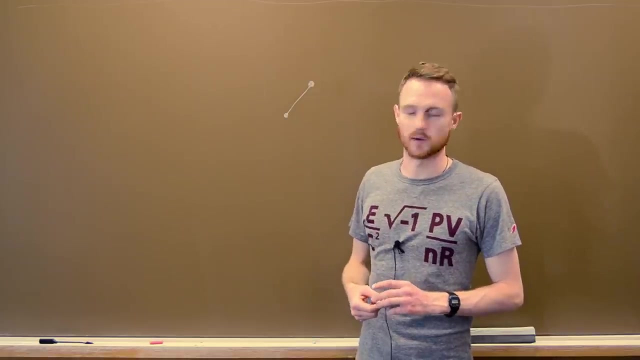 Homo-morphically irreducible trees of size n equals 10.. So what does that mean? That's all the information they gave you in the movie. So, first level of clue, let's just explain what those terms mean. A tree is a combination of points which will draw us circles and connections, dots and lines, whatever you want. 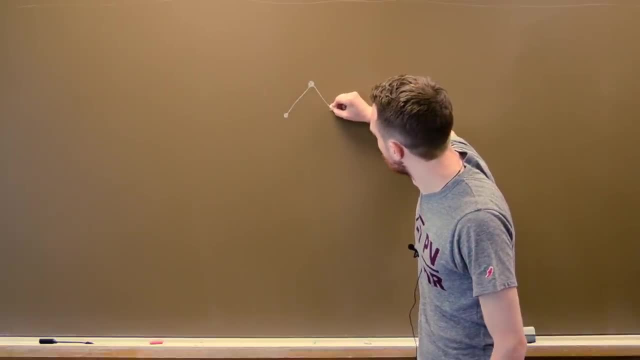 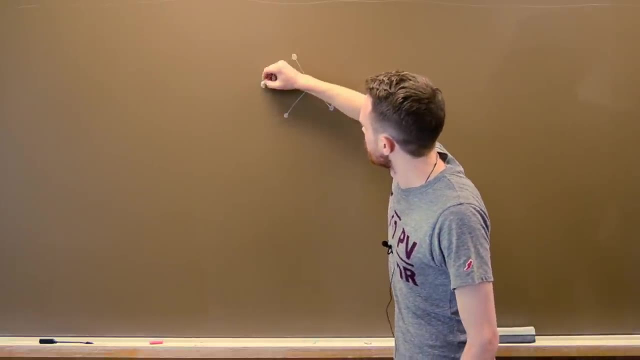 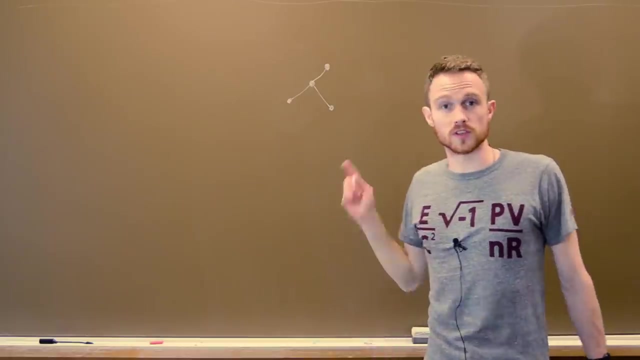 So this is a tree. This is a tree. What's not Allowed with these trees is loops. So you can't have this point connecting here. making a loop, It's not allowed. So this is a tree. of size n equals four. 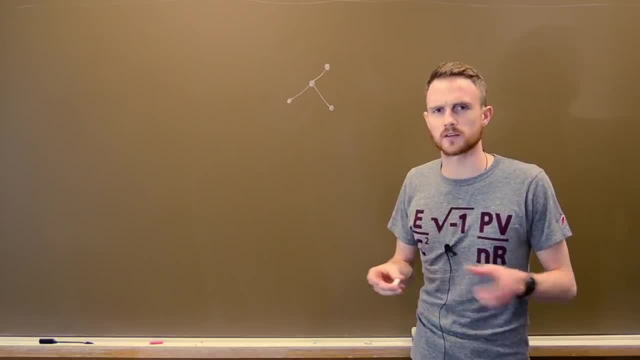 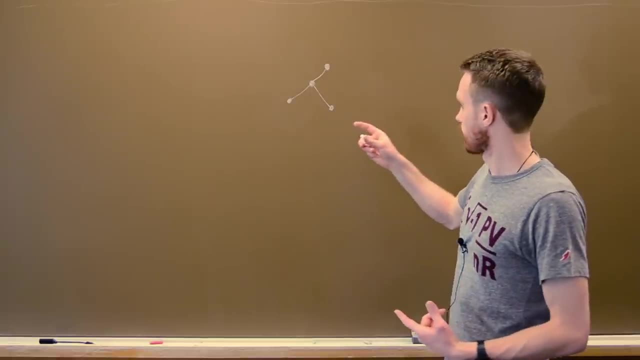 There are four dots of four nodes in this tree. Now let's look at the other words in that homeomorphically. What does that mean? So let's say I draw another tree. This is a tree of size. n equals six. 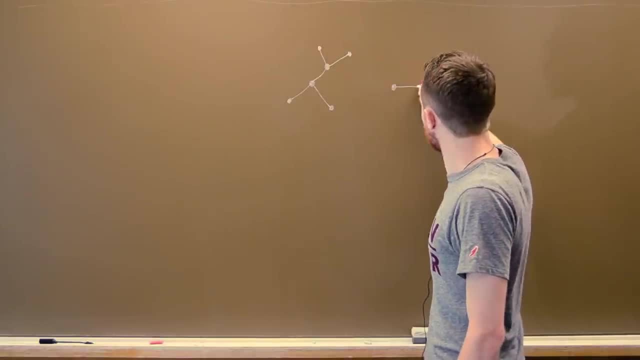 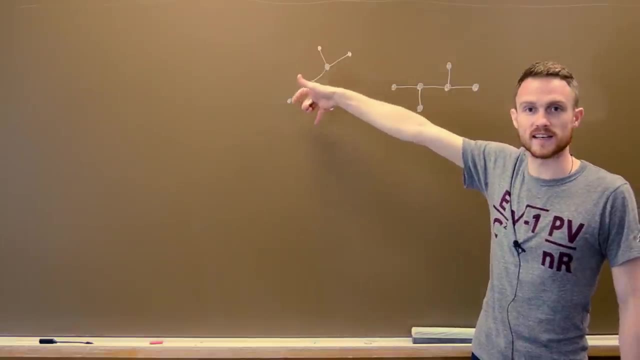 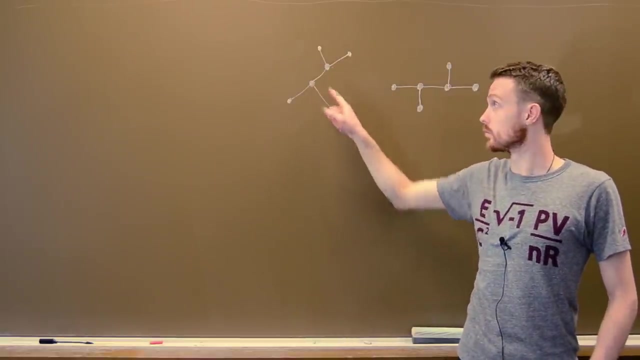 Now were I to draw another tree, these are effectively the same tree, So you can see. it's more or less just me rotating this around, maybe changing the angle slightly, but which points which nodes are connected to which other nodes remains the same between the two. 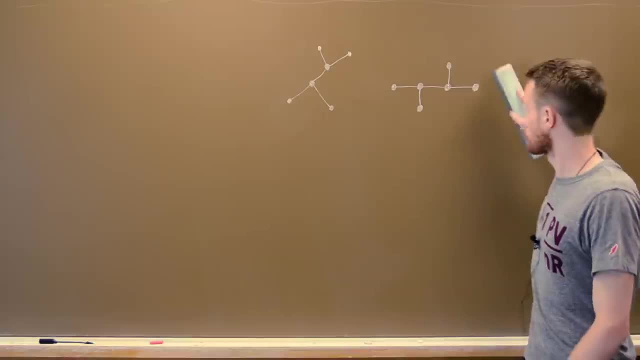 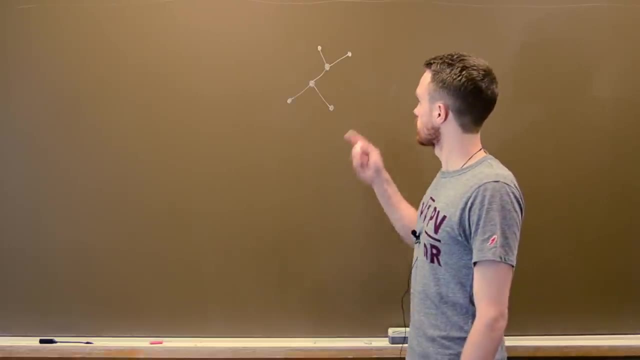 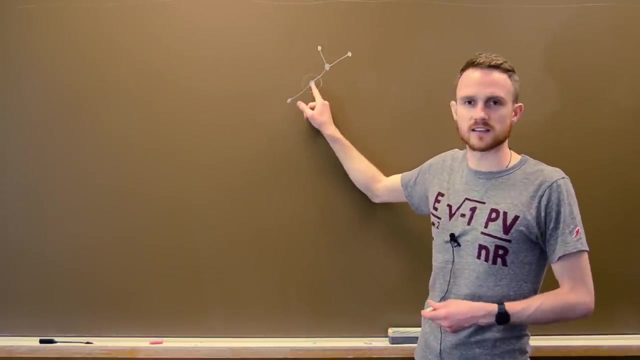 So these are not unique. This only counts as one tree. So that's the homeomorphic part. What about the irreducible part? So let's say, I didn't have this node here, This point here. when you get to this node, say you're coming along here. you get to this node, you only have one option. 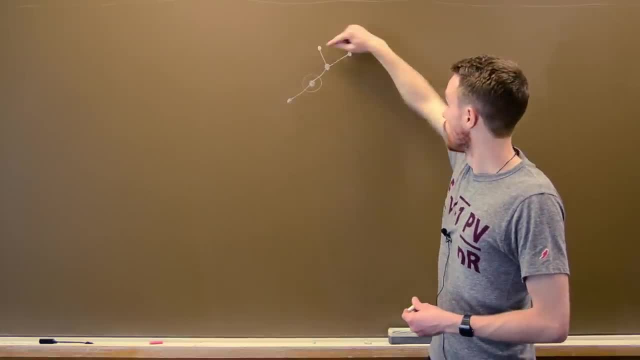 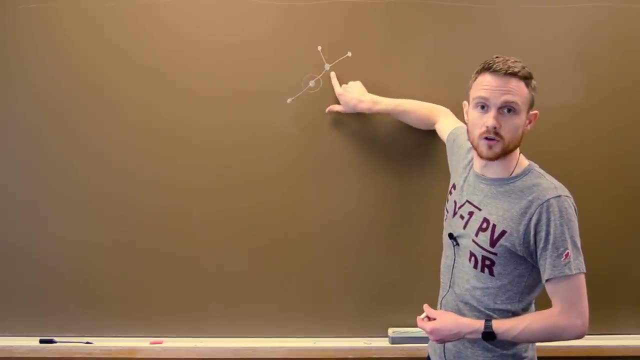 Then it's not irreducible. So here you can see if I come down from this point. I have two options and go over this way or down this way. This is okay. This is a node that's allowable. The only ones where you can connect one option are the end nodes. 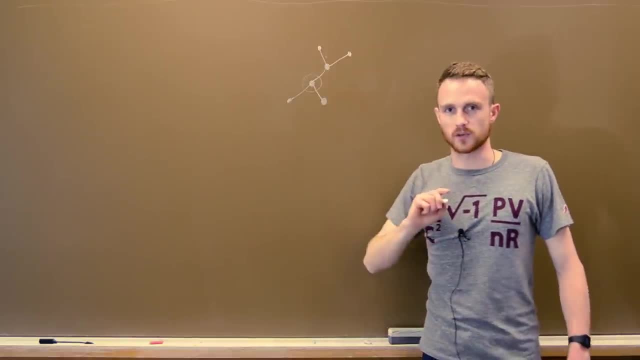 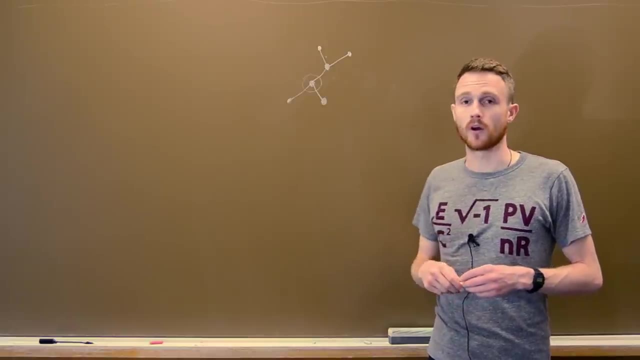 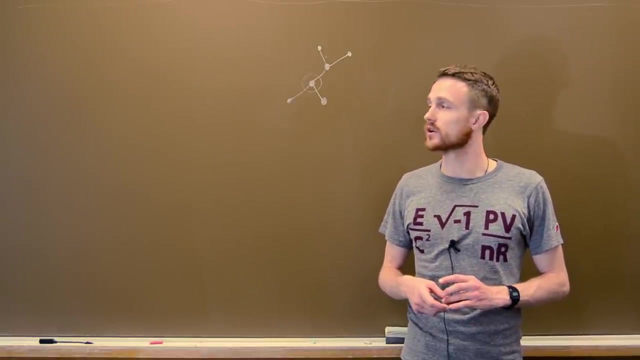 So this is banned, But that's okay. So those are the rules. Only homeomorphically irreducible trees of size n equals 10.. The next clue I'm going to give is the number of trees in the solution. So remember, you have to draw all of them, but you don't know at this stage how many there will be. 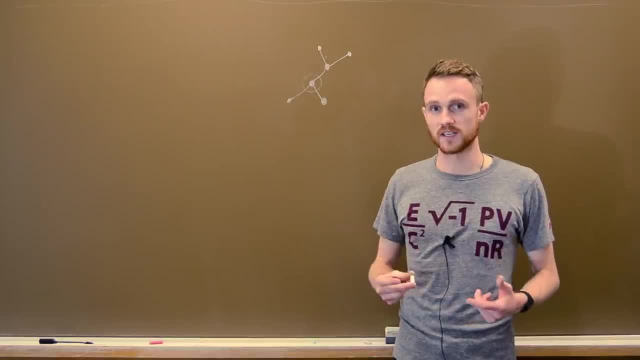 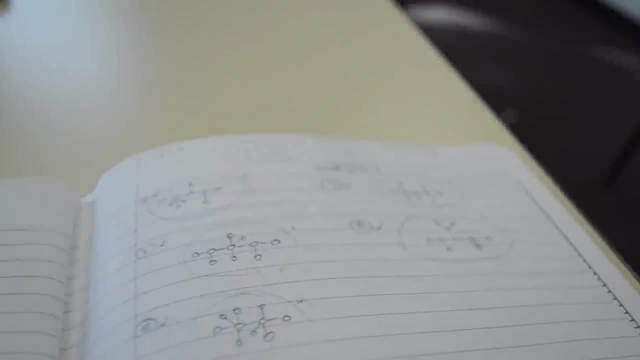 You don't know at what point to stop. The number of trees in the solution is 10.. We know we have to draw 10 of these trees, But deciding what's unique, What's homeomorphic, can be tricky, Especially once you start getting to large trees. 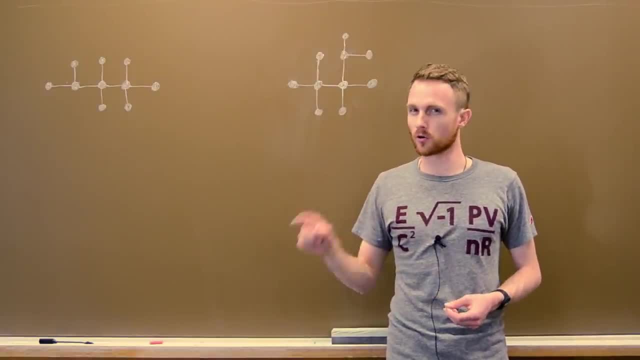 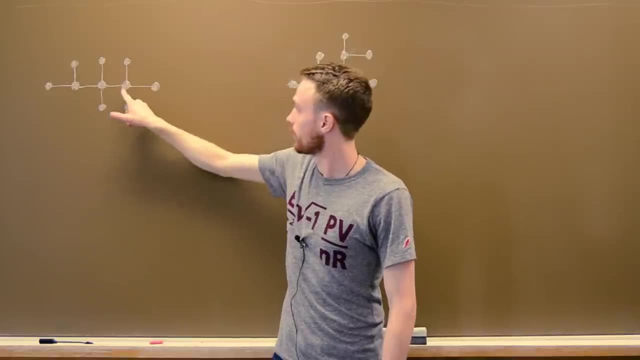 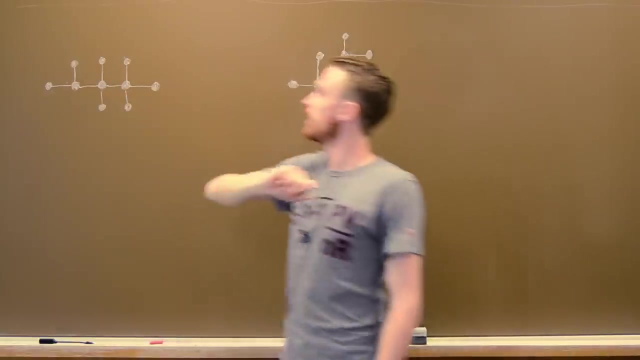 One good way to keep track of this is to ask yourself what is the longest chain in the tree. So here we have 1,, 2,, 3,, 4, 5.. It's pretty easy. You could go 1,, 2,, 3,, 4, 5 up here or down here, or this way. 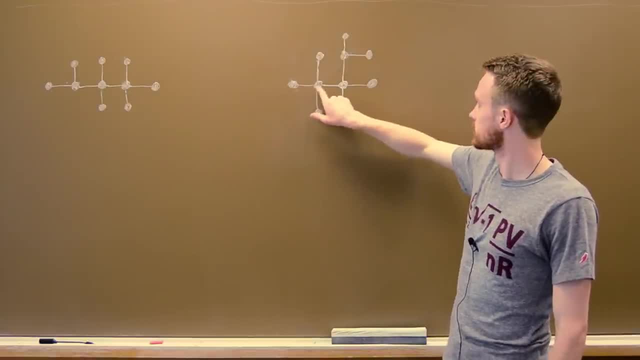 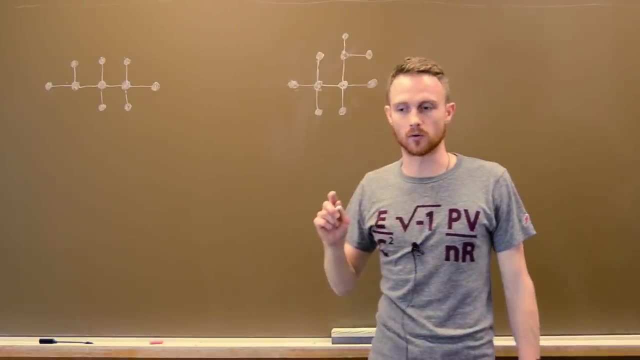 And our longest single chain in here is also 5.. So 1, 2, 3, 4, 5, or 1, 2, 3, 4, 5.. What you can do, then, is to number the number of branching nodes that come off of each of the middle nodes in the tree. 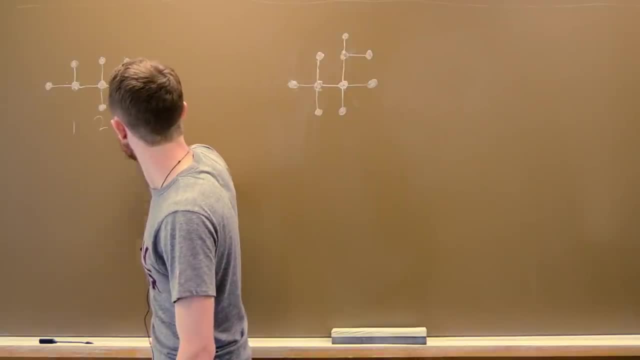 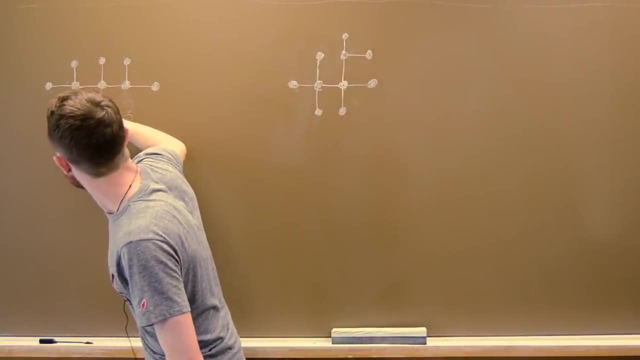 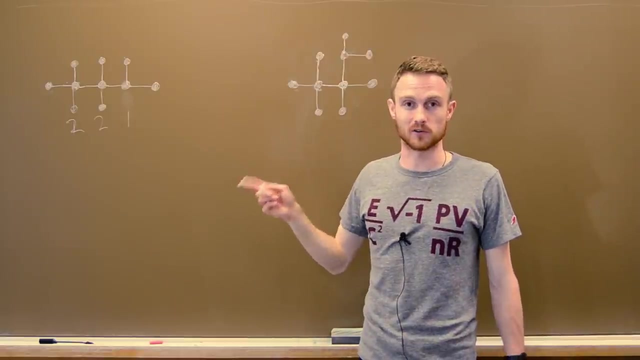 So we've got 1 coming off of here, then 2, then 2.. Note that if I move this over here- And that became 2. And that became 1.. That is also the same tree That is not homeomorphically irreducible from the other one. 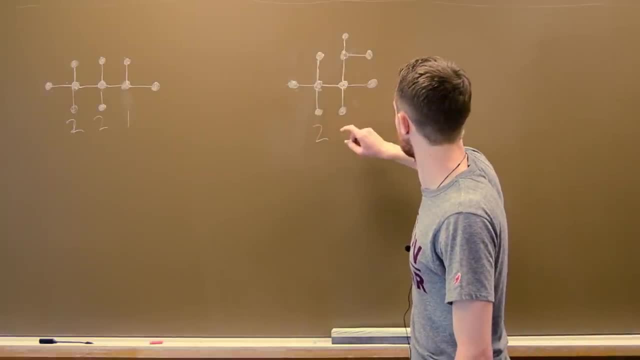 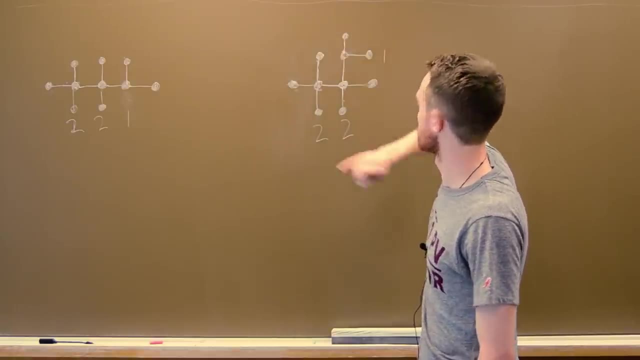 And here we can look at this. We have 2.. We have 2 coming off of the next one And off of this one we have 1.. Not counting the end node, So ignoring the end nodes, you have 2, 2, 1, 2, 2, 1.. 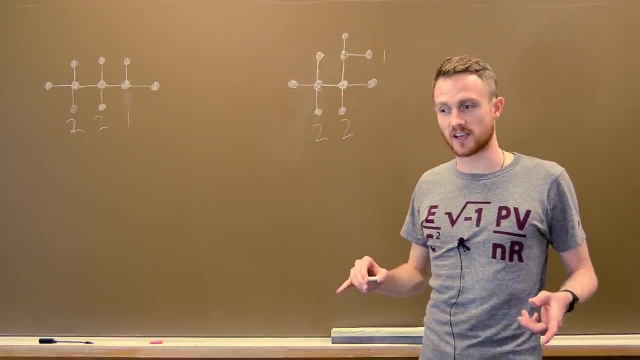 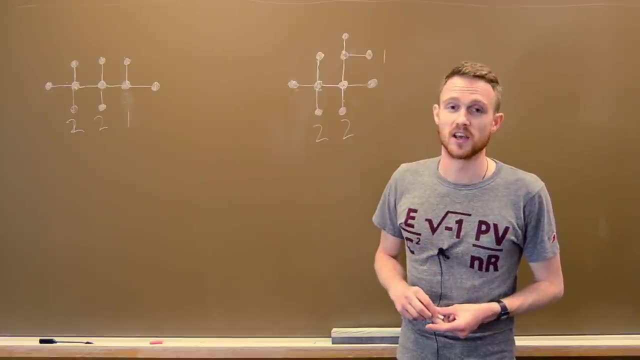 It's the same tree. So use this technique to think about what those 10 different trees are. So let's see what the answer is. If you want to solve this problem yourself, and I highly recommend you do, now is a good time to pause the video. 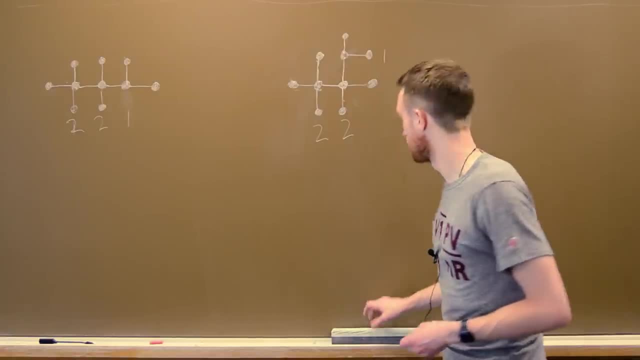 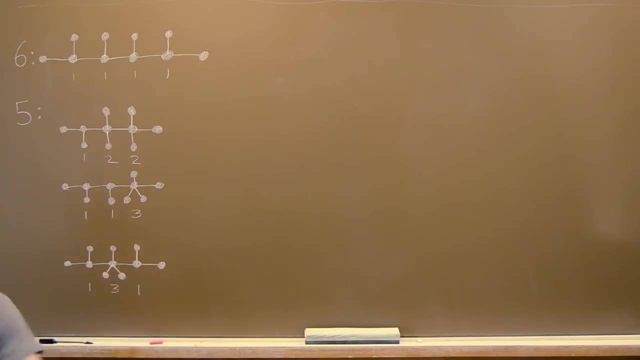 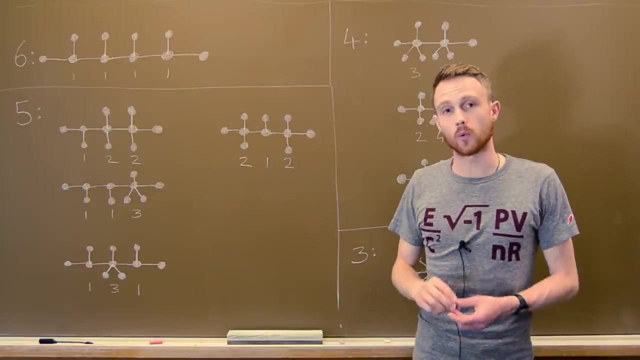 But we'll get the answers up here in just a moment. Okay, So, using our numbering convention of looking at the longest single chain in the tree, We have 4 different lengths of tree that we can have: 6,, 5,, 4, or 3.. 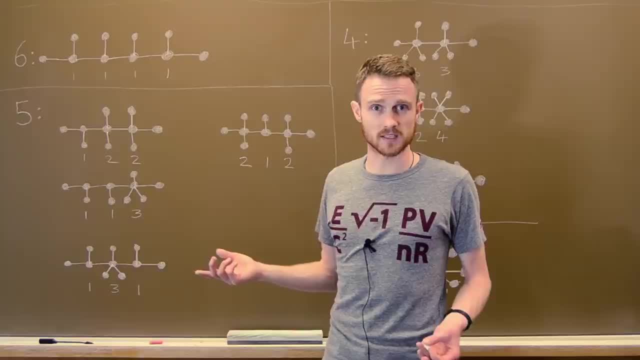 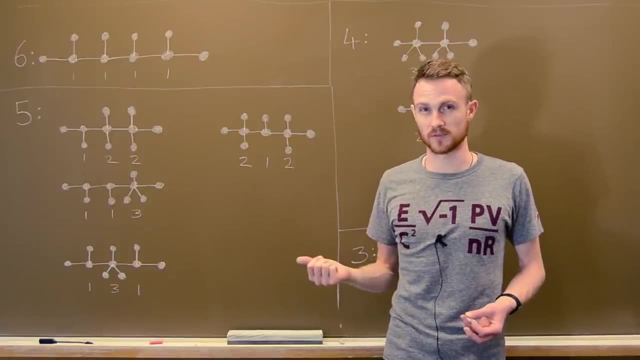 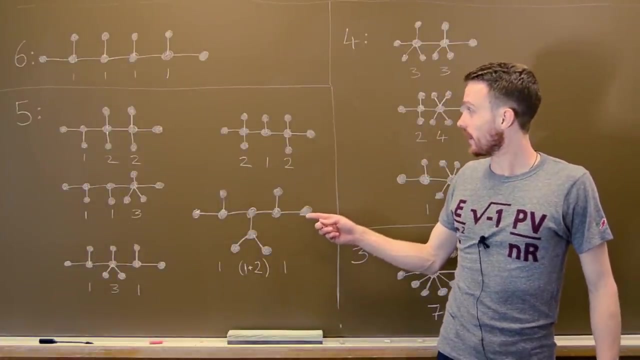 We notice here that, though I said before that there were 10 solutions, right, There's another one, And this is where the numbering convention that we've used here kind of falls apart. Okay, So in this last solution here Previously, all other solutions. 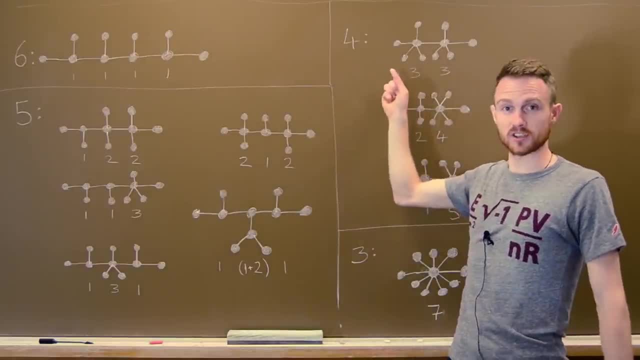 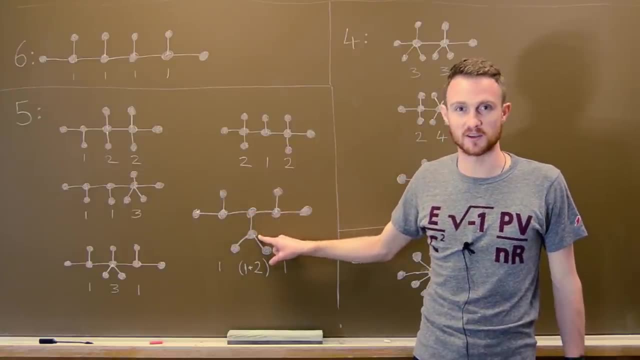 You could point to one of the middle nodes, And each of the end nodes connects directly to that. But here we have a middle node with a second middle node connected to it, Or rather a third middle node connected to it, And it's allowed. 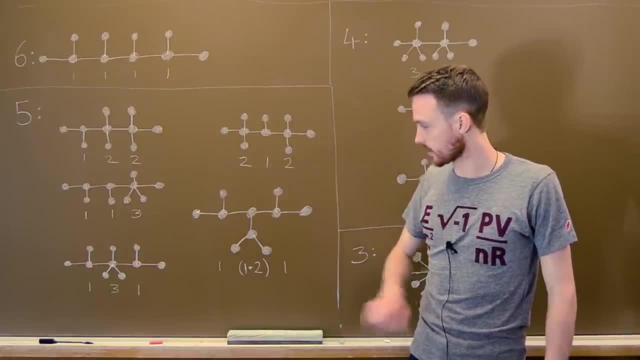 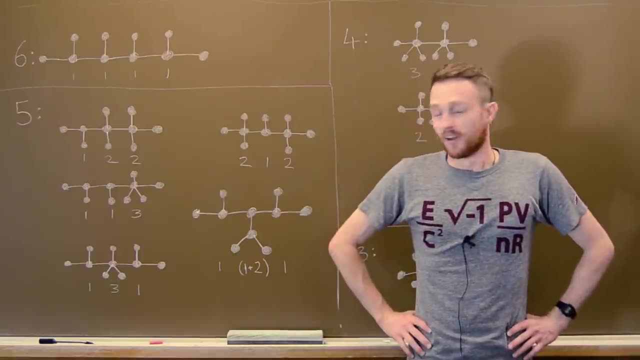 You know we're coming into here. It's still a junction. You have 2 options, So I like to call this 1, 1 plus 2, 1.. So that's it, You know, Not as difficult. I don't think it would have taken an MIT professor 2 years. 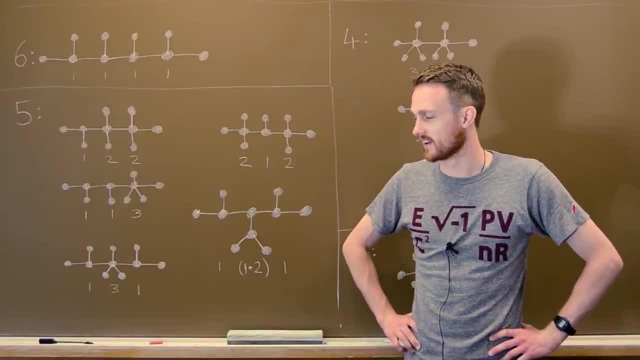 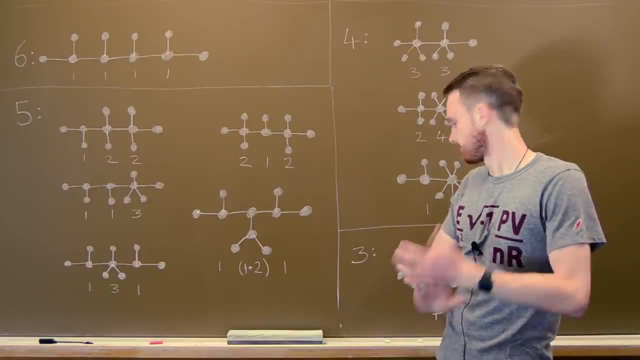 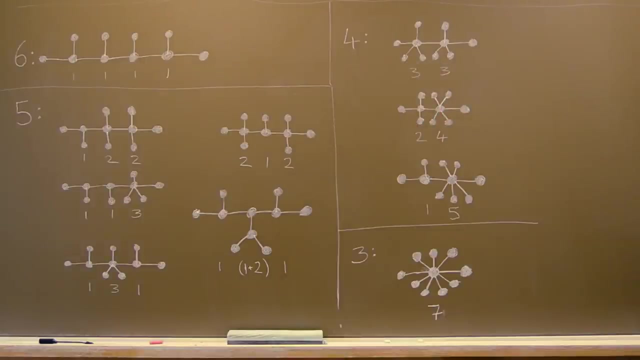 Hopefully this is something that you had fun solving, And I know I did So. now you can tell yourself that you're as smart as Will Hunting, Who's a fictional character. So you may be wondering: why doesn't this look like it does in the movie? 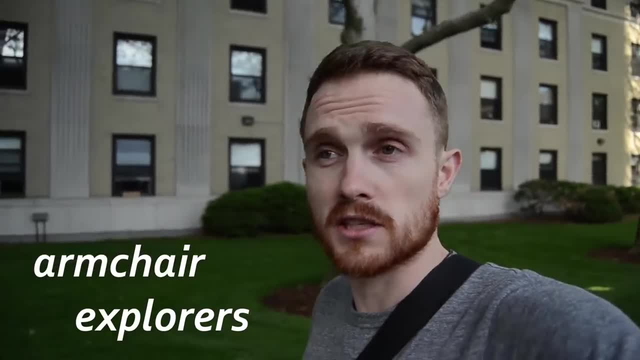 Why couldn't he find the same chalkboard? The answer is that a lot of the film was actually shot in Toronto. 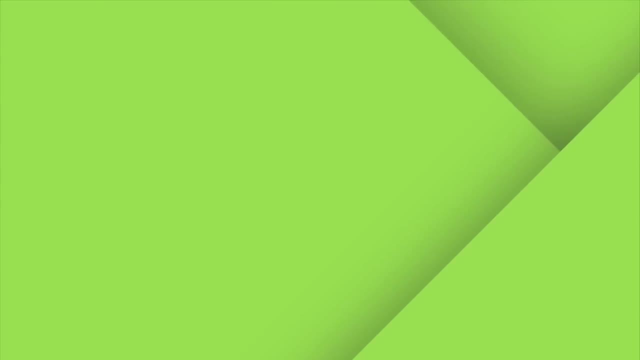 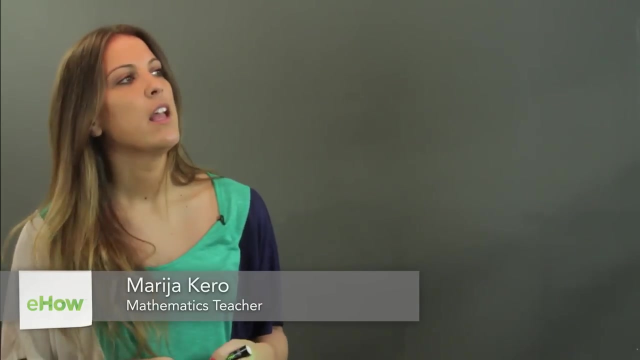 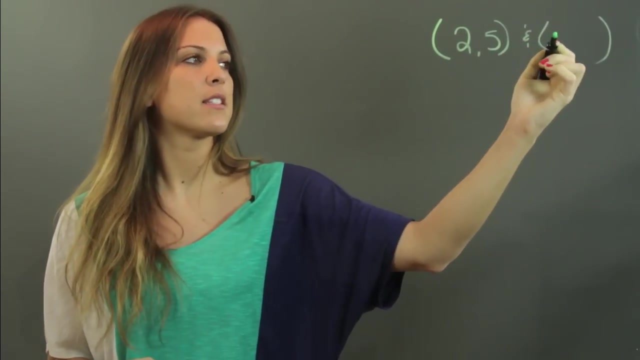 Hi, my name is Maria, I'm a mathematician and today I'm going to show you how to write a linear equation when you're given two points. So if I'm asked to write the equation of a line that goes through the points 2,, 5, and let's say 4, 9.. 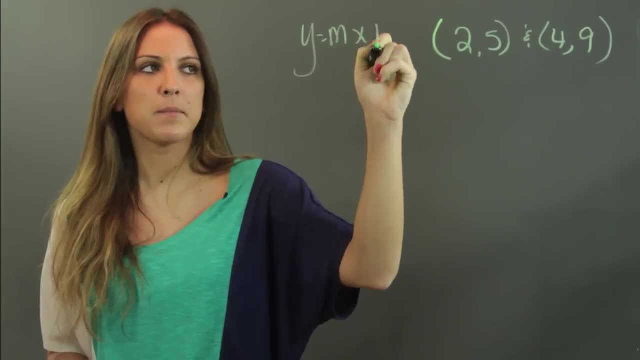 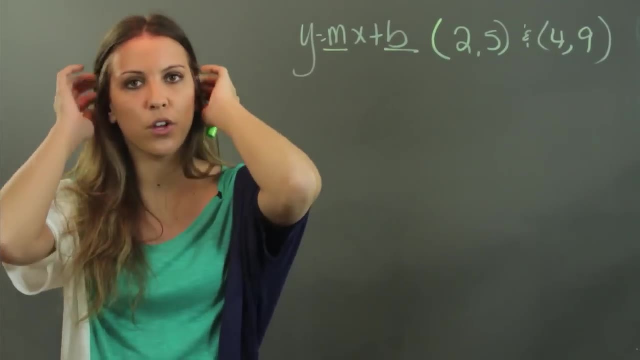 The first thing you should write down when you're asked to write an equation is: y equals mx plus b, the slope-intercept form of a linear equation, And what you need to know is that m and b are going to have to get filled in in order for your equation to be complete. 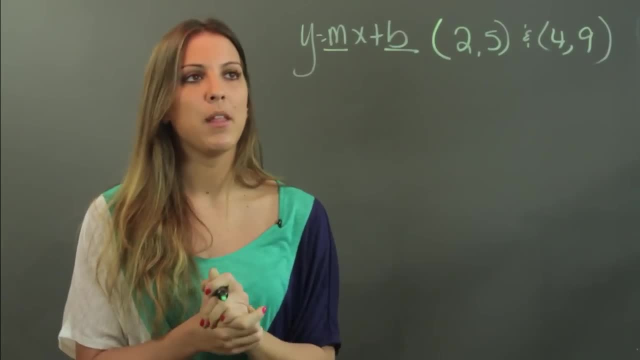 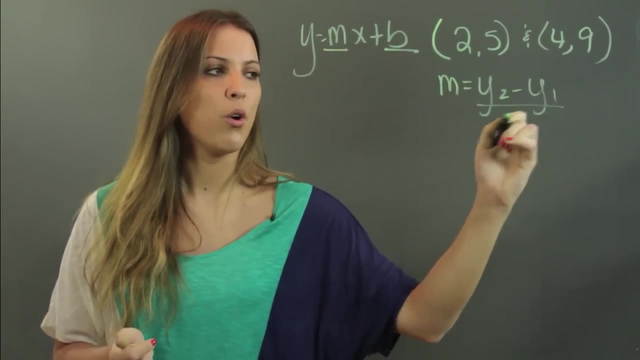 So now you have to ask yourself: how do you find m and how do you find b? Well, m is your slope, so you have to know the slope formula, which is: m equals y2 minus y1 over x2 minus x1..